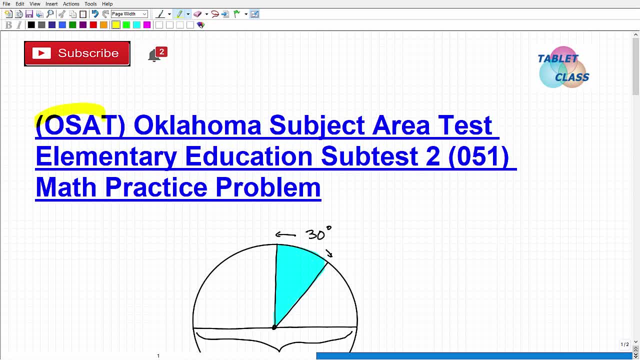 Okay, let's talk about the OSAT, or rather the Oklahoma Subject Area Test, but we're going to be talking about a specific test, and that's the Elementary Education Subtest 2, and this is the code here- 051, for that particular OSAT test, and it has to do with math. 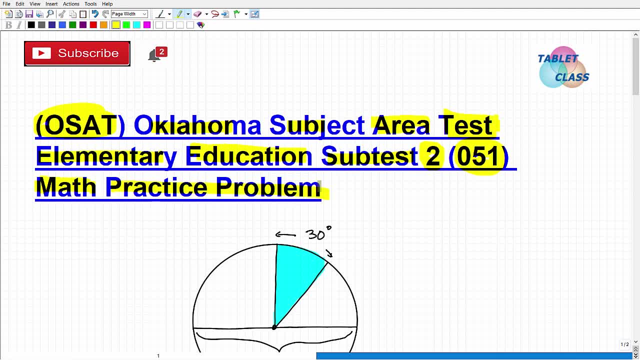 So we're going to be taking a look at a math practice problem that you should be able to handle if you expect to do reasonably well on this Subtest 2, on this particular OSAT exam. So we'll get into this problem here- a nice little challenging problem here in a second. but let me introduce myself. 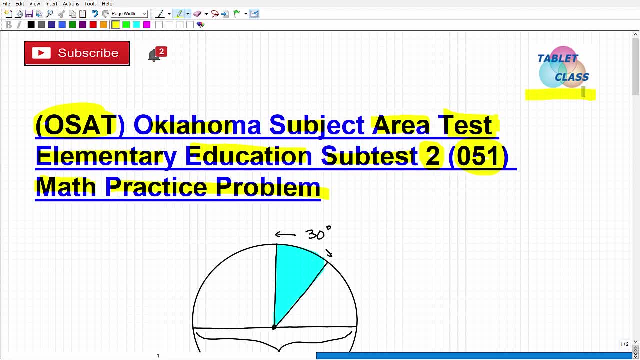 My name is John. I'm the founder of Tablet Class Math, middle and high school math teacher, so I know what it's like to take certification exams, teach in the classroom, go to college, get a master's degree- All of the above. so everything that you're doing I've done as well, and so I certainly appreciate all the effort it takes to become a teacher, irrespective of what level you're at. 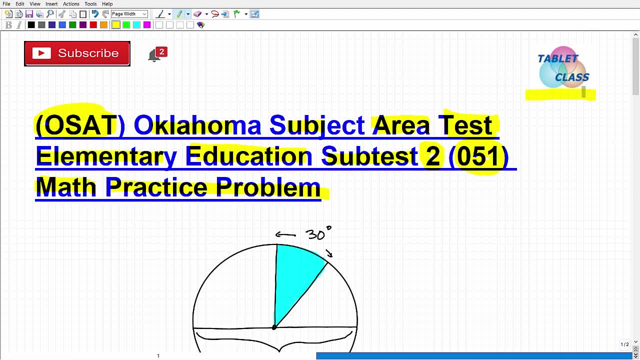 High school math teacher to elementary level doesn't make a difference. All teachers have to put in a lot of effort to get their license and teach. So anyways, with that being said, I do want to say that what I do is I construct a lot of courses. 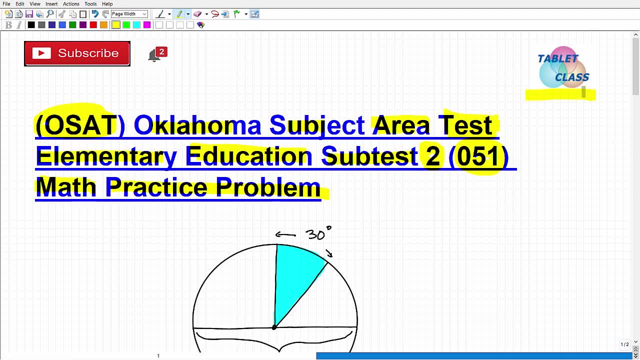 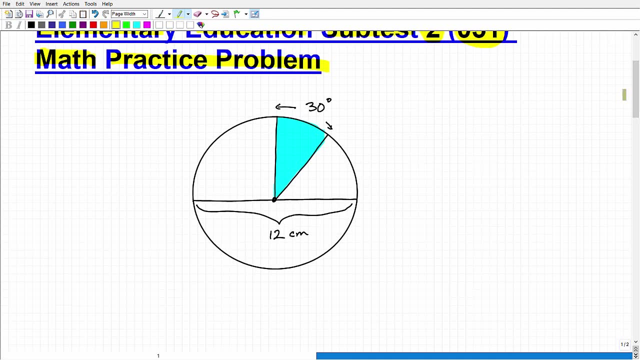 I've been doing this for many years: online math courses. Actually, I have a very comprehensive math prep course for this particular exam. I'll leave the link to that in the description of this video. but what I want to do is kind of challenge you to take a look at this particular problem. 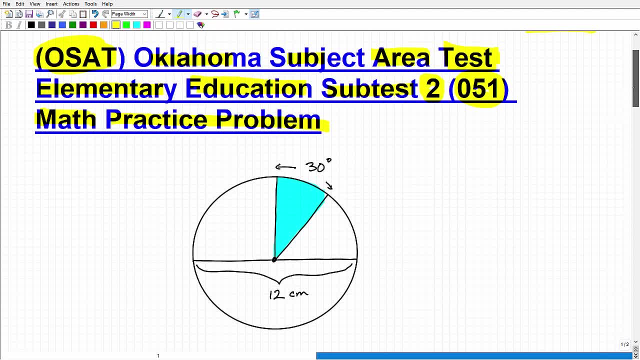 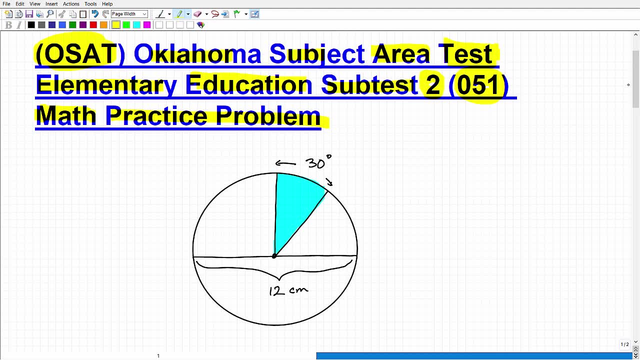 because this is the kind of level of math that you're going to be expected to know on this OSAT exam. So one thing, especially with elementary teachers, that if you don't really look at what's going to be on the exam, it's not just elementary math okay. 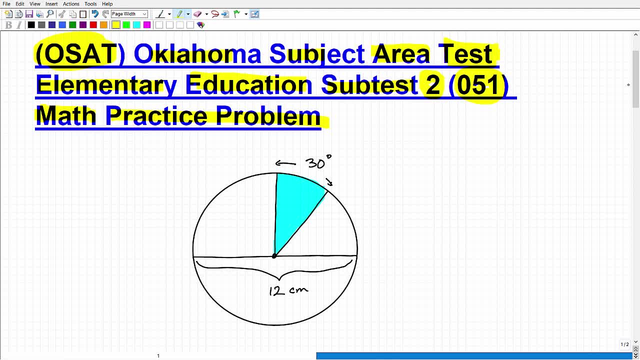 So, although you're going to be at the elementary level, the math that you need to know for your certification is- I kind of classify it as high school level math, so a good amount of algebra, geometry and other subjects as well. So you really have to study for the exam and, as you know, people do fail these certification exams. 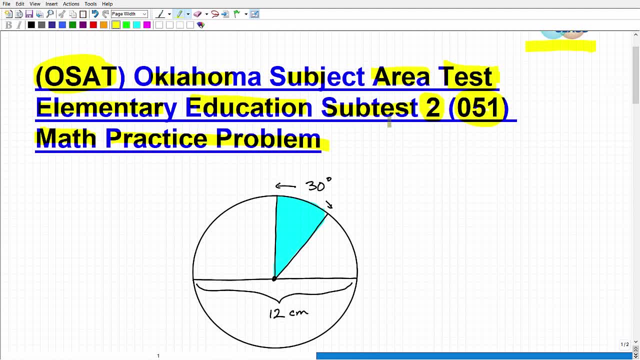 It's not uncommon for teachers to have to take a lot of effort to do that. So you really have to take these exams more than once. so you don't want to be in that position if you can avoid it. So you know the smart thing to do is prepare in advance, and if you kind of struggled with math, or even if you're good at math, 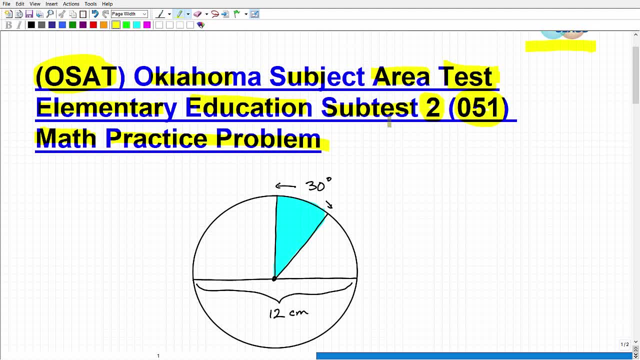 like let's say, you know you took a math course two, three years ago or back in high school. you're like: oh, I was good at math and I don't really have to do too much studying. I don't think that's a good approach, okay. 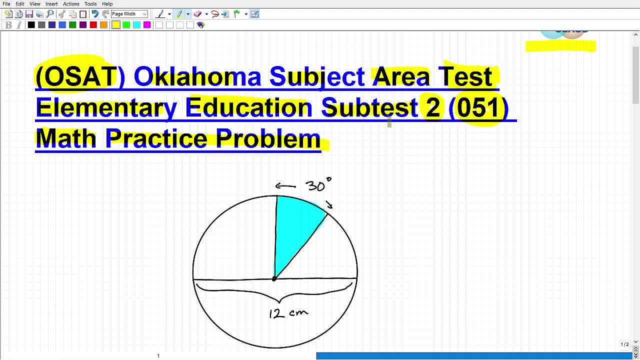 Even if you're strong in math, there's a lot you have to recall, Okay, so you really have to do a lot of studying and brush up on things so you can walk into this exam confidently, and that's the whole idea. 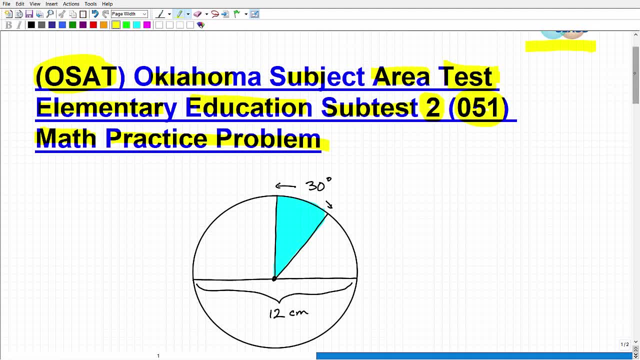 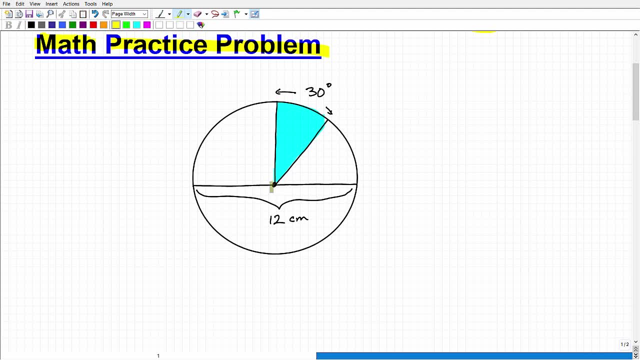 It's better to over-prepare than under-prepare, for sure. Okay, so let's get to this problem. Let me explain what's going on. So here we have a circle, and this is emanating here from the center. It may not be perfect. 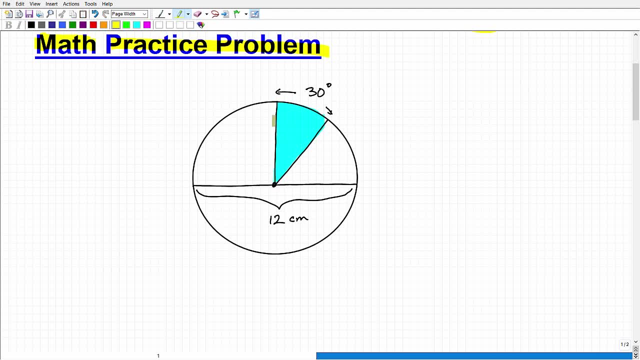 It's kind of a rough sketch. So from the center of the circle I have this little pizza pie, this little sector we call, and it goes like this It goes. it's basically 30 degrees wide right here, this arc. 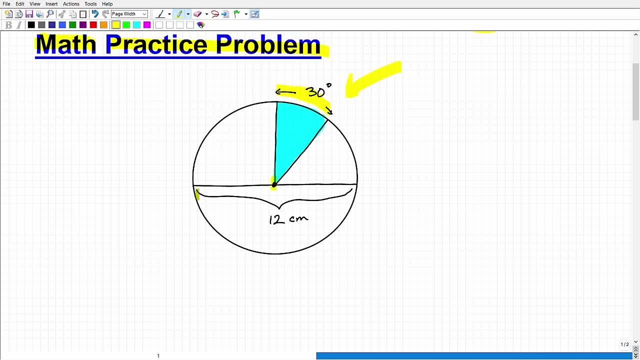 Okay, so this forms this sector from the center, and then this is the width of the circle. We also call that the diameter, So it's 12 centimeters wide and you have this information here. What I'd like you to do is find the area okay of this sector. all right, this little pizza slice. 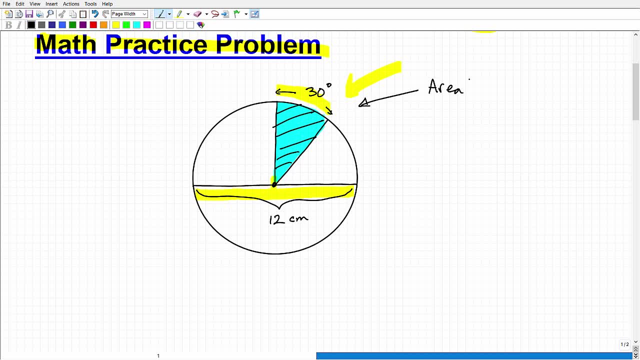 So find the area, if you can. Now I'm going to kind of give you a clue here. I'm going to give you the formula that you need to solve this problem, and then, of course, I'm actually going to solve it. 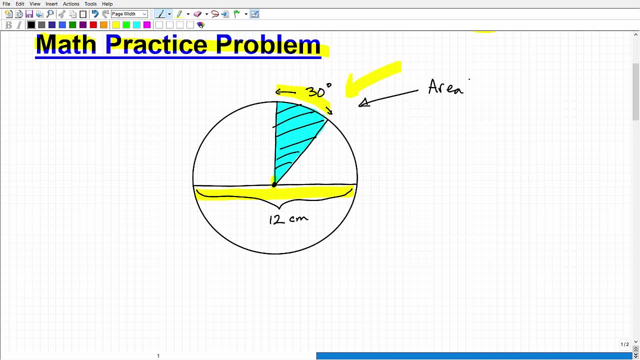 But I'm just curious to see if you remember what formula to use. Okay, so if you want to pause the video and try to recall that formula and then solve the problem, that would be excellent. Okay, so, before I actually solve the problem completely, 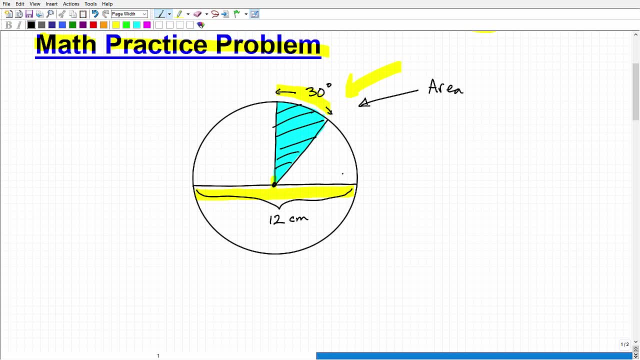 the one thing you need to know is the area of a circle. Okay, The area of a circle is pi r squared, All right, so hopefully you remember what the r is. Okay, And now let's go ahead and get into solving this problem. 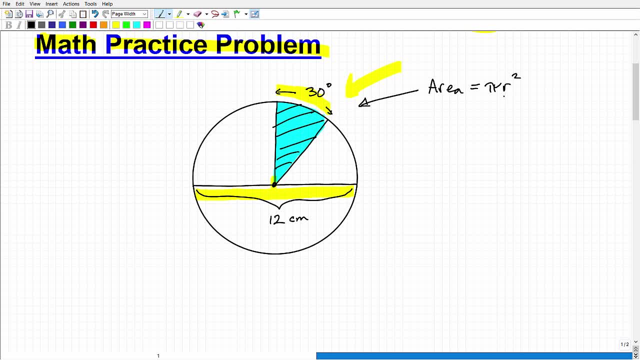 Now, of course, any time you want to pause the video and do it yourself, I certainly encourage that. But there's a couple things here, right? So we have this is the formula for the area of a circle and we have this sector right. 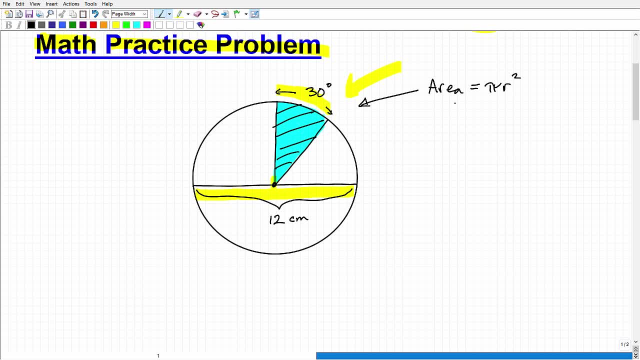 So we want to find the area of this sector, not the entire circle. But let's just see how we're going to first find the area of the entire circle and then we'll get to this sector part first. So the area of the entire circle is equal to pi r. 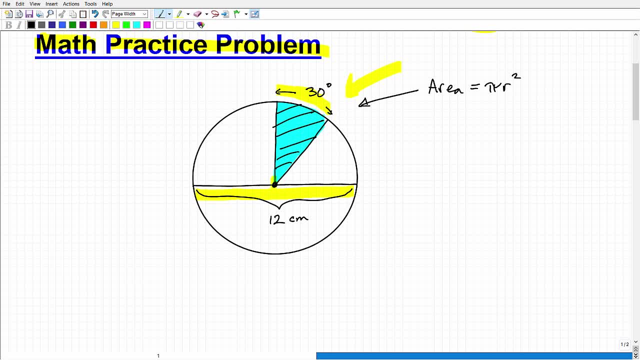 r is the radius. The radius is the distance from the center of the circle out to the edge of the circle. So in this case it would just be half the diameter, or 6 centimeters. Okay, So hopefully you knew that. So let's go ahead and just find the area of the circle real quick. 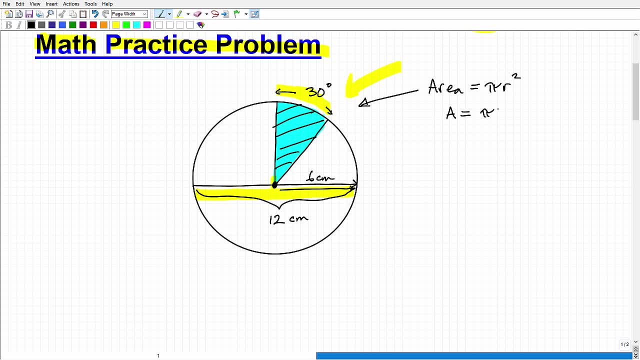 So the total area of the circle is going to be pi. The radius is 6.. I'll get to the units of measure here in a second right And that's going to be squared. So 6 squared is 36.. And then we'll write this pi behind that. 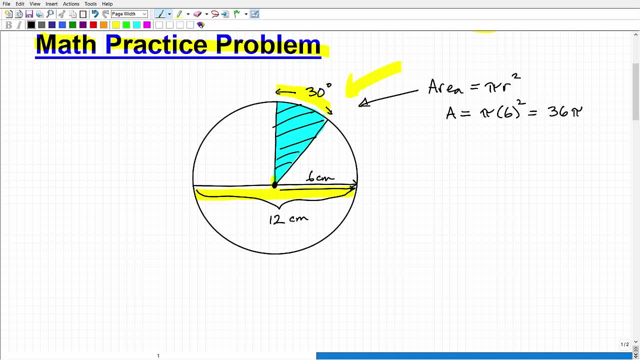 So this is the way you would write that: 36 pi. Now we are using the units of measure of centimeters, So it's going to be centimeters squared, So that's the area of the entire circle. But I don't want the area of the entire circle. 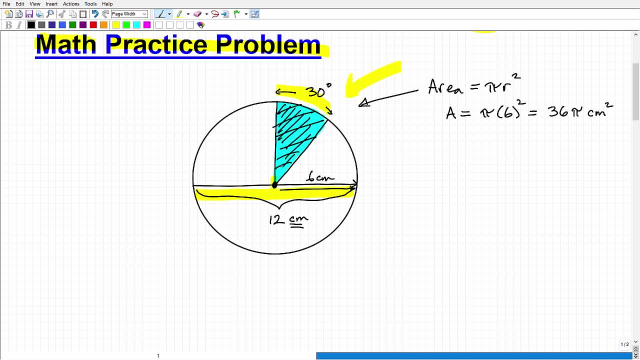 I want the area of this particular little segment of it. Now, the way we're going to figure this out is: notice that this is 30 degrees. Okay, This arc right here is 30 degrees. Well, you kind of need to basically set up a little ratio here. 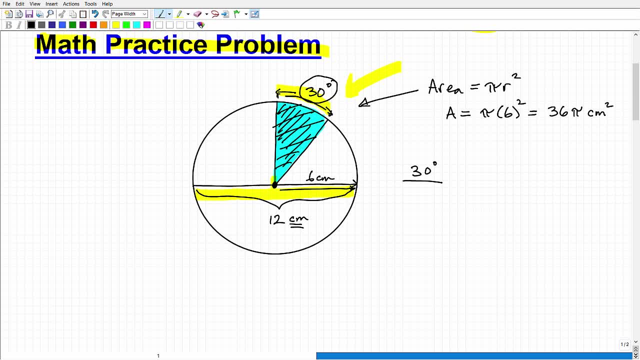 Okay, That this is going to be 30 degrees out of the entire distance around a circle, Okay, Or a measure, And that's 360 degrees. So really we're just finding the area of this proportion here right: Just 30 degrees out of the entire 360.. 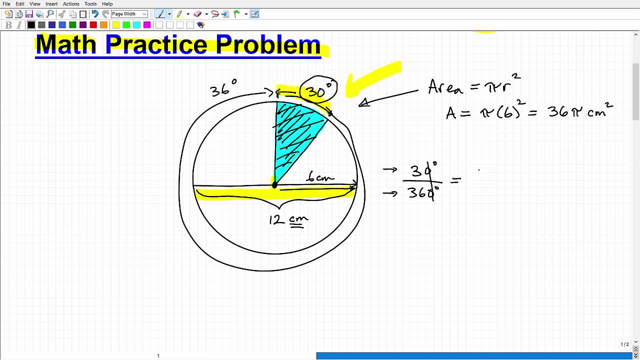 So that is going to be. let's go ahead and just reduce this fraction. That's going to be 3 over 36, or 3 goes into 36, 12.. So we're going to be finding the area of 1 twelfth of the circle. 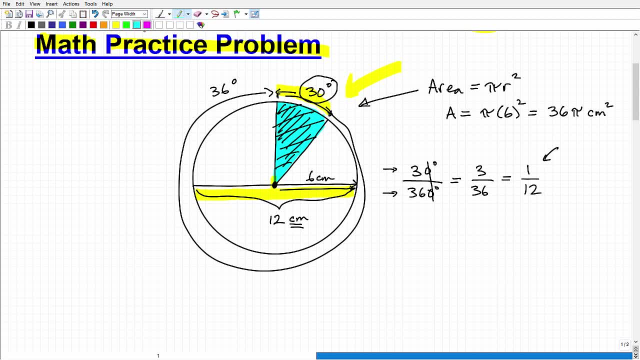 Okay, So this is what we're actually looking for. Okay, 1 twelfth of the circle, So we have the area of the entire circle. Okay, So we just need to find 1 twelfth of the area of that entire circle. 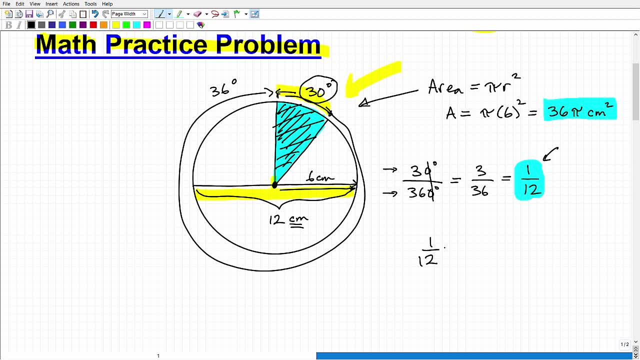 So let's go ahead and do that now. So that's 1 twelfth times. Let me write that a little bit better. So 1 twelfth times 36 pi. We'll get to the units of measure in a second: 36 pi. 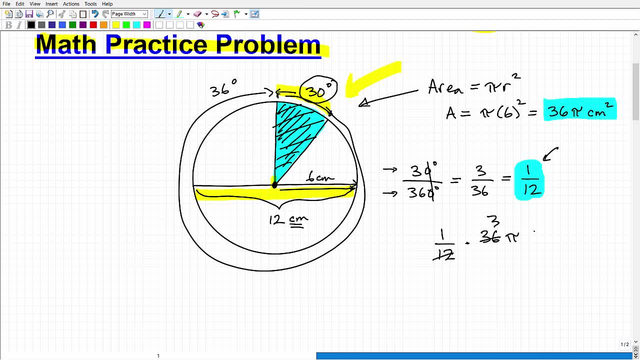 So 12 goes into 36. That would be 3.. So this would be 3.. 3 pi centimeters squared. Okay, So that is the answer. That's the area of that circle, And if you got that right, that's excellent. 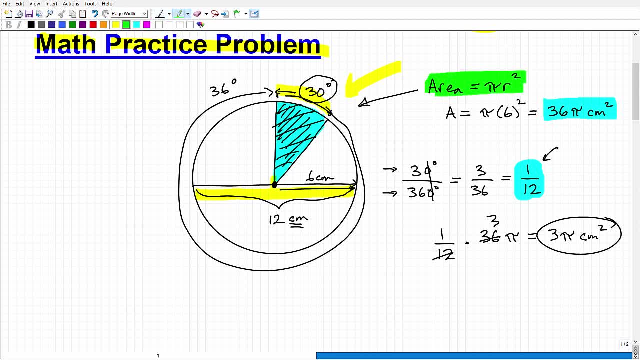 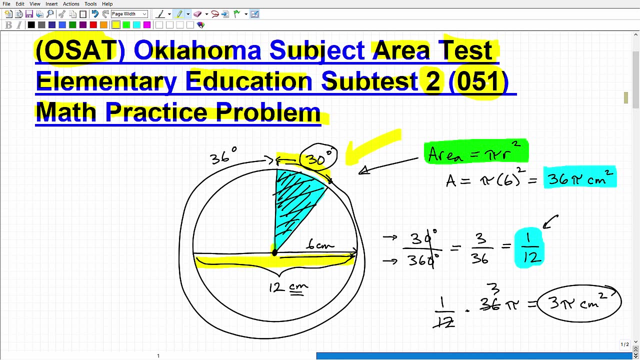 Okay, Especially if you remember what formula to use. So this is a basic level, high school level type of geometry problem, Something for sure that you should be able to handle on this particular exam. Okay Again, especially at the elementary level. as I said, most elementary school teachers- oftentimes, if you don't really take a look at what's on the exam, you think it's just going to be like place value and fraction. 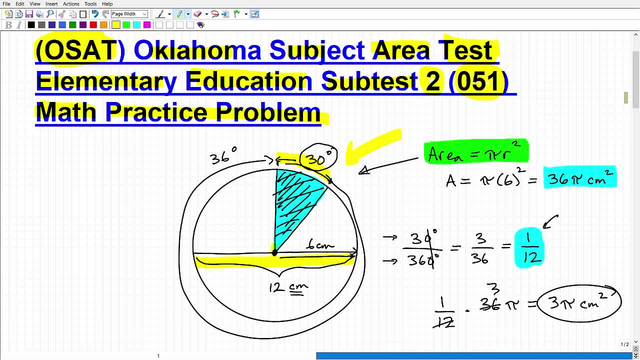 You know things you're going to be actually doing at the elementary level, But it's not the case. Okay, You're always going to be, you know, tested at a higher level. So, for example, the middle school level for math, you know you really need to know more advanced high school level math and beyond. 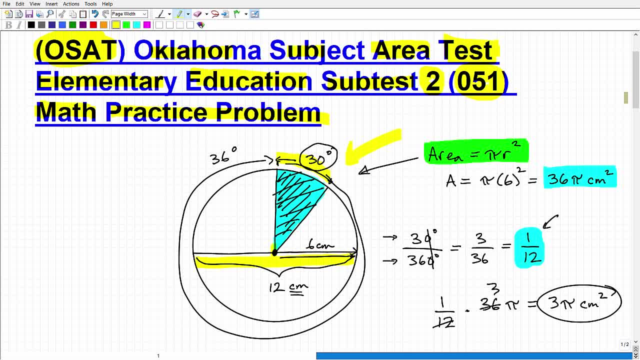 And at the high school level you have to get into. you know more advanced math than that. you know calculus et cetera. So it's just the way it is. So hopefully you know again. if you got this right, that's excellent.